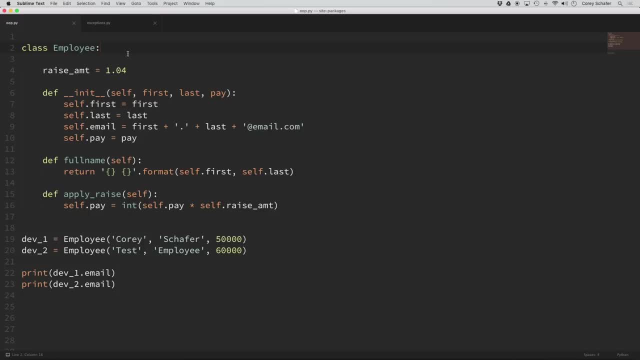 class. Now let's say that we wanted to get a little more specific here and create different types of employees. So, for example, let's say that we wanted to create developers and managers. Now, these will be good candidates for subclasses, because both developers and managers are going to 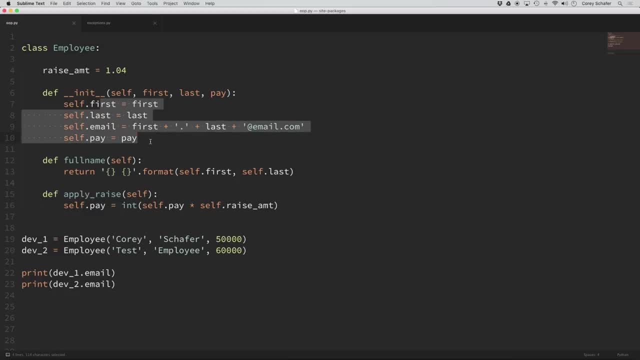 have names, email addresses and a salary, and those are all things that our employee class already has. So instead of copying this code into our developer and manager subclasses, we can just reuse that code by inheriting from employee. So let's go ahead and create these developer and manager subclasses. 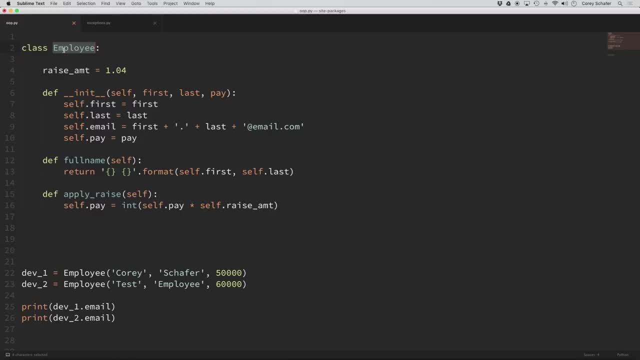 And it's just as easy as creating a new class, just like we did up here with employee. but we're going to call this new class developer And after the name of the class we can put these parentheses here and specify what classes that we want to inherit from. 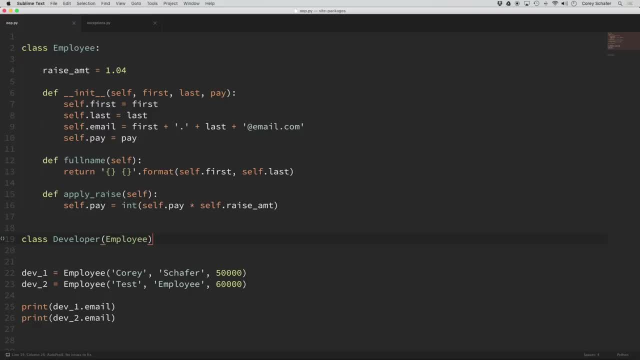 So in this case we want to inherit from developer And in this case we want to inherit from the employee class. Now I'm just going to put in this past statement here for now, because I want to show you that by simply inheriting from that, 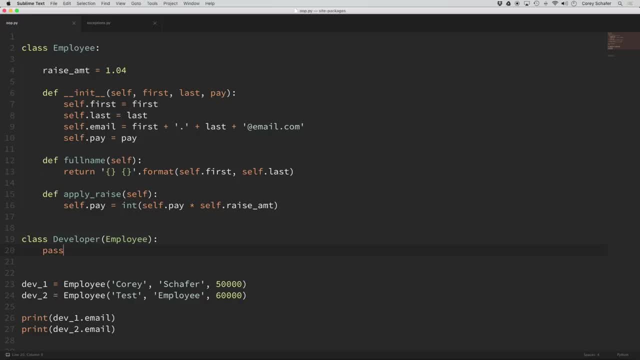 employee class that we inherited all of its functionality. So right now, even without any code of its own, the developer class will have all of the attributes and methods of our employee class. So right now, down here I have two instances of our employee class, and then I'm 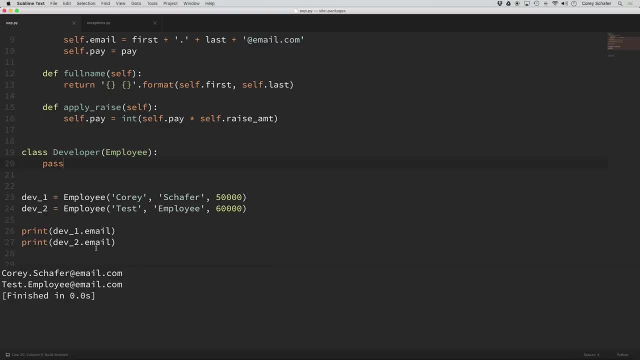 printing out both of their emails. So if I save this and run it, you can see that when we create two instances of our employee class, we're going to have two instances of our employee class. So if I save this and run it, you can see that when we create two instances of our employee class, 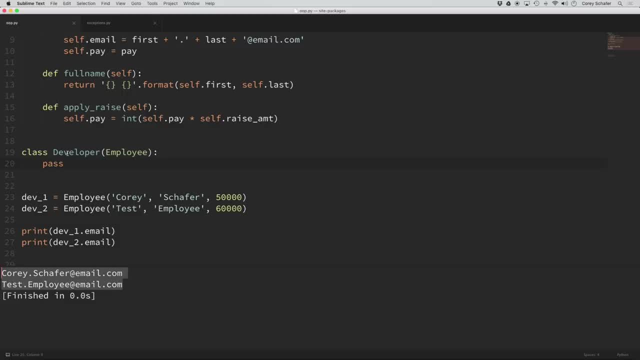 we're going to have two instances of our employee class. So if I run this and print out their emails, that we get this result. So now, instead of creating two new employees, I'm now going to create two new developers and pass in all of the same information. So now, if I rerun this and 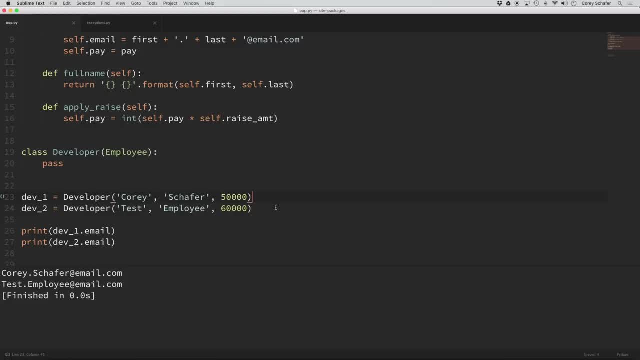 print out those emails, you can see that those two developers were created successfully and that we can access the attributes that were actually set in our parent employee class. So what happened here is that when we instantiated our developers, it first looked in our developer class and then 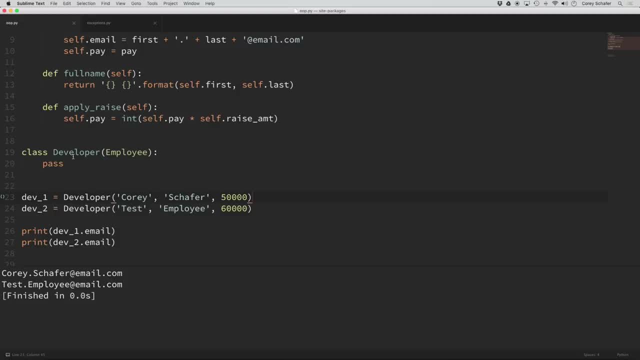 it looked in the class for our init method, And it's not going to find it within our developer class because it's currently empty. So what Python is going to do, then, is walk up this chain of inheritance until it finds what it's looking for Now. this chain is called the method resolution. 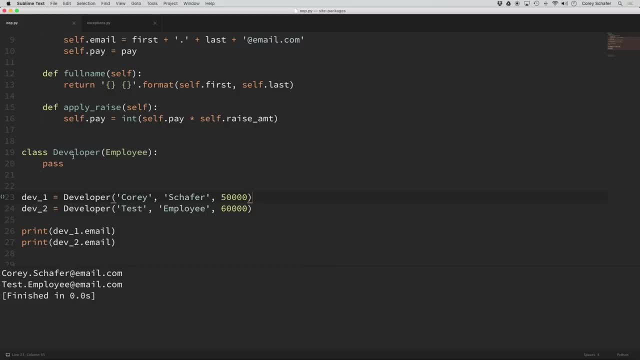 order. Now I want to show you this really useful function here that makes these things a lot easier to visualize, and that is the help function. So first I'm going to copy out these two lines here, and then I'm just going to print out this help function. 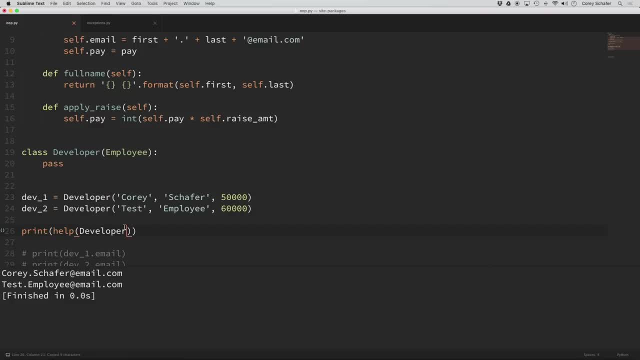 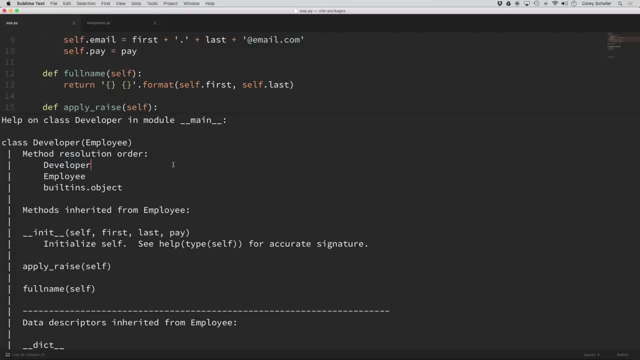 And I'm going to pass in the developer class. So if I go ahead and run that and I'm going to make this a little bit bigger here Now, you can see that when we run help on that developer class that we get all kinds of good information here. So that method resolution order that I mentioned. 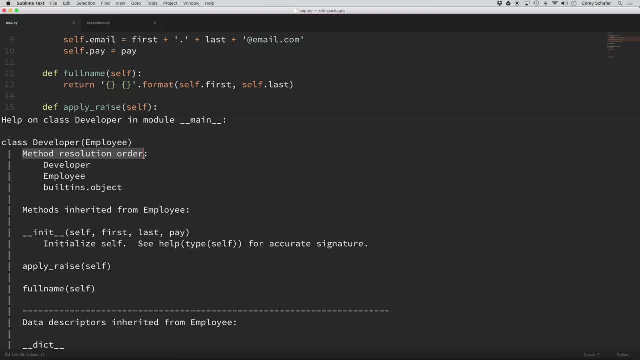 is one of the first things that gets printed out, And basically these are the places that Python searches for attributes and methods. So when we created our two new developers here, it first looked in our developer class for the init method, And when it didn't find it there, then it went up. 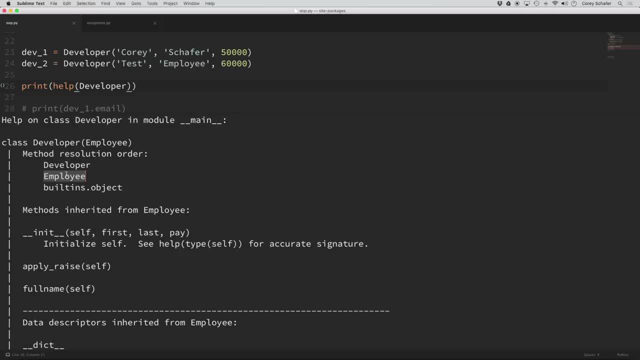 to the employee class and it found it there, So that's where it was executed. Now, if it hadn't found it in our employee class, then the last place that it would have looked is this object class, And every class in Python inherits from this base object. Now, if we look at this output, 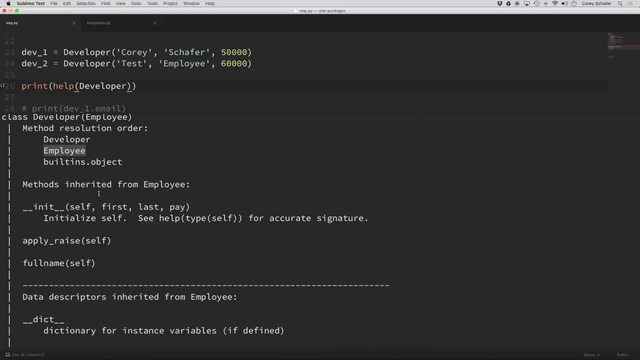 further, then it actually shows the methods that were inherited from employee. So you can see here that we have the init method and we also have our employee class And if we look at this output, our apply raise method and our full name method, And if I keep scrolling down here, then you can. 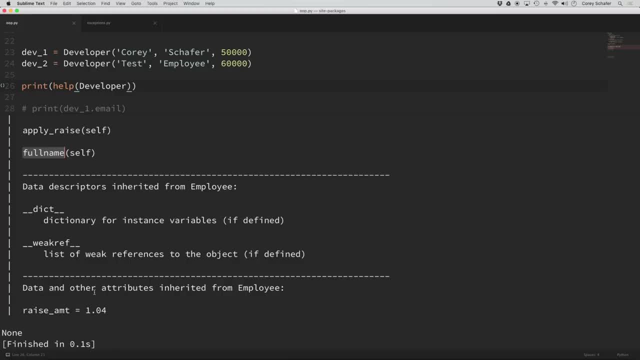 also see that we have our data and other attributes, And you can see that the class attribute, raise amount, was also inherited from the employee class. So we got all of this code for free just by inheriting from that employee class. Okay, so now I'm going to go ahead and make this. 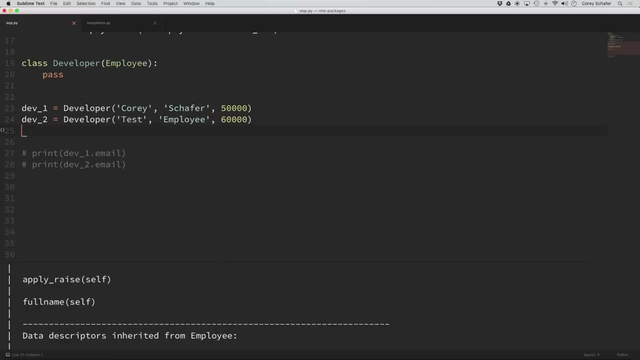 smaller again And I'm going to take out that printed help statement. Okay, so now let's say that we wanted to customize this And we're going to take out that printed help statement. It's going to tell us: And I'm going to take out our data And I'm going to take out our subclass a little bit. Now I'm 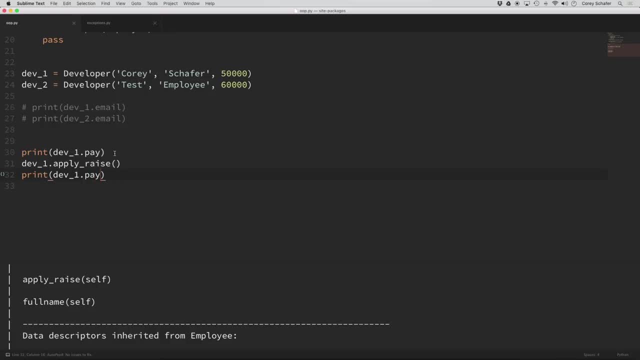 going to make a very simple one line change in here And I'm just going to change the raise amount. But first let's go ahead and see what happens when we apply a raise on our current developer. should find our employees raise amount of 4% and that I'm going to reprint out. 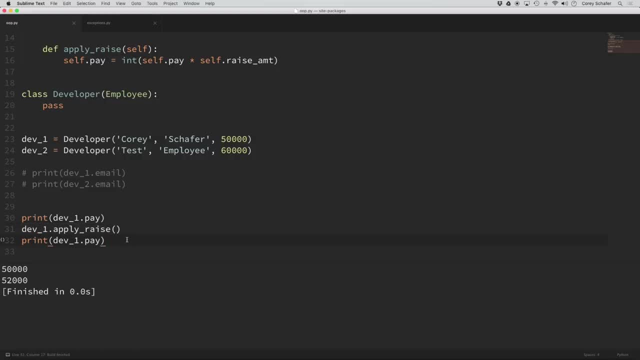 that developers pay again. so if I save that and run it, you can see that it printed out 50,000, applied the raise and then printed out 4% higher. but let's say that we wanted our developers to have a raise amount of 10%. now to change that. 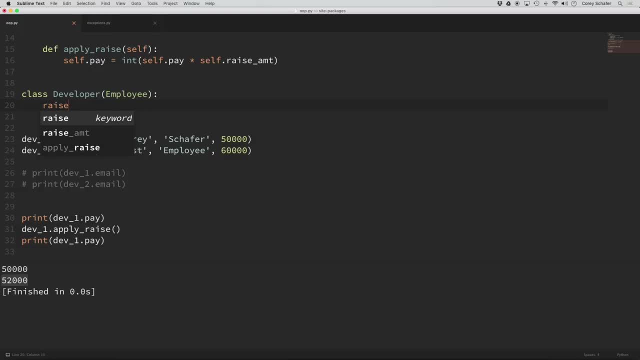 it's just as easy as coming into our developer class here and changing the raise amount to 10%. so now, if I go ahead and rerun this, you can see that it used our developer classes raise amount instead of our employee classes raise amount. now, if I was to change this instance back to an employee instead of 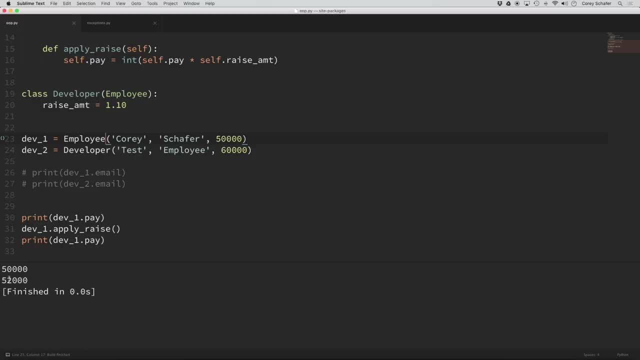 a developer and then rerun this, then you can see that now it's back to that employee 4% amount. so the thing to take away here is that by changing the raise amount in our subclass, it didn't have any effect on any of the classes that we were using in our developer class. so now, if I go ahead and 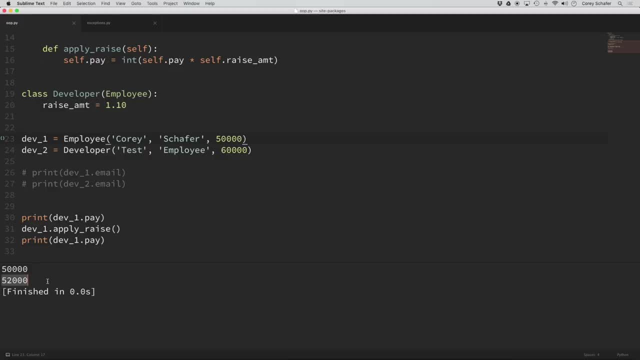 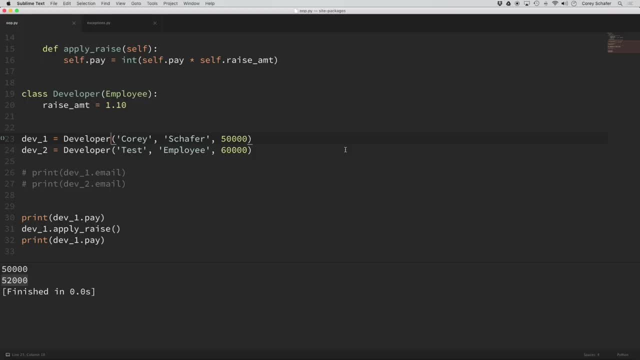 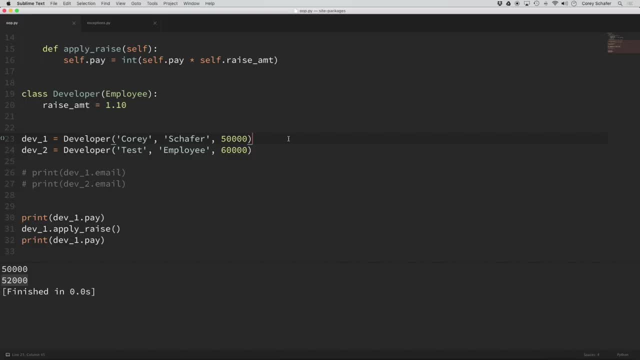 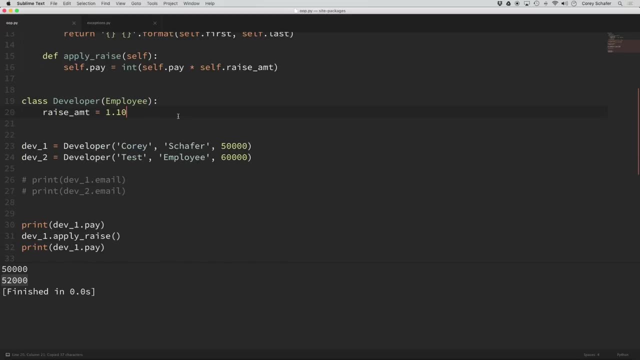 around this. we're going to have to give the developer class its own init method. so what I'm going to do is I'm just going to go up here to our employee class and grab that init method and I'm going to paste it here within the 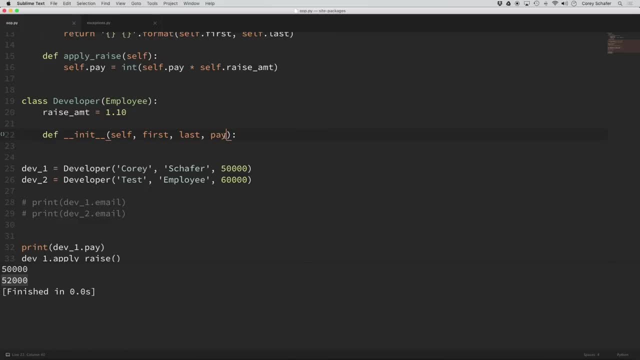 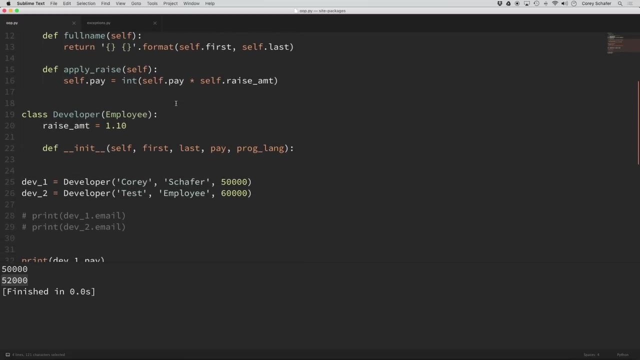 developer class now, along with the first name, last name and pay. I'm also going to add in an argument here for the programming language. now what you might be tempted to do here is just go up and copy all of this code from our employees classes init method and paste it into our developer classes init method. but 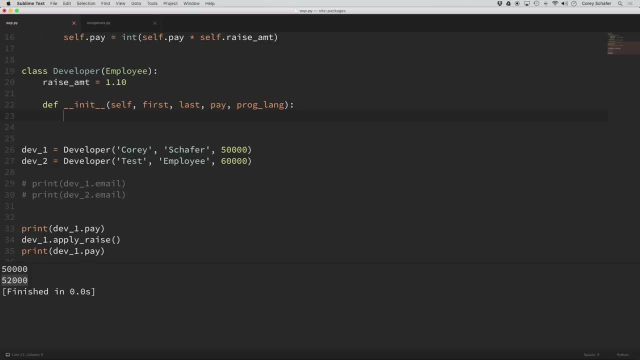 we don't want to do that because we want to keep our code dry and not repeat this logic in multiple places, because we want it to be as maintainable as possible. so, instead of copying and pasted, pasting that, what we're instead going to do is just let our employees and init method handle. 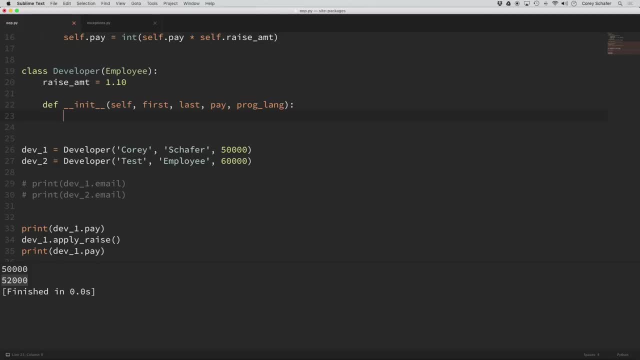 the first name, last name and pay, and then we'll let the developer set the programming language. so, in order to let that employee handle the first name, last name and pay, what we can do here is just do super dot and knit and then we can pass in the 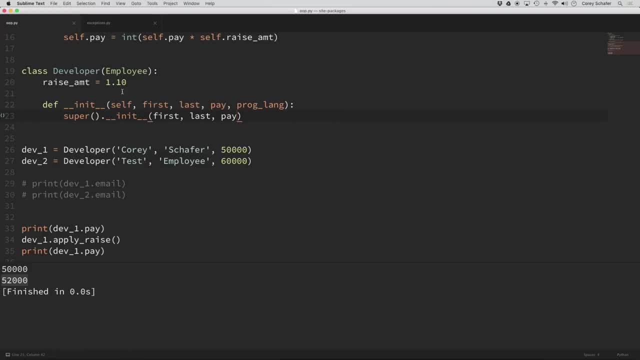 first, last and pay. So again, superinit is going to pass first, last and pay to our employee's init method and let that class handle those arguments. Now there's multiple ways of doing this logic here. You may have seen some people do employeeinit and instead of passing in first, 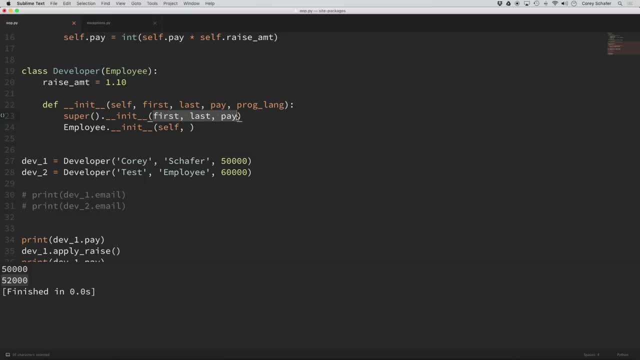 last and pay. they'll type in self and then first last and pay. Now, both of these ways of calling the parents init method will work, but I tend to use super because with single inheritance, like we are using here, it's a little bit more maintainable, but it's really necessary once you start using. 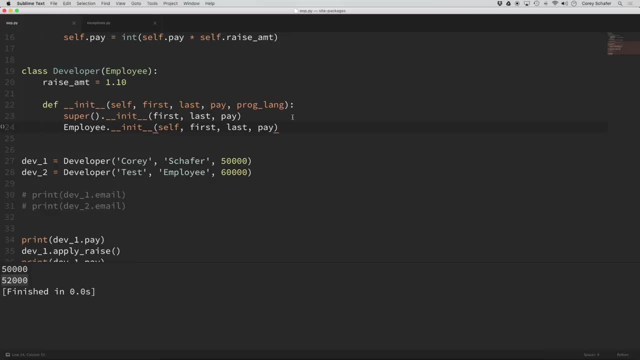 multiple inheritance and we're going to go over that in a future video. But to keep things simple, I usually just like to always stick with super. So now that we're letting our employee class, as init method, handle the first, last and pay, now we can handle the programming language. 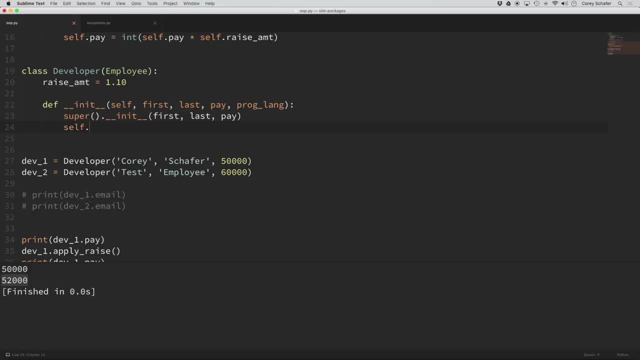 argument, just like we would in any other class. So I can just say: selfprogramminglanguage equals the programming language that we passed in here. Okay, and that should be all we need for our init method. So now, when we instantiate our developers down here, it's also going to be. 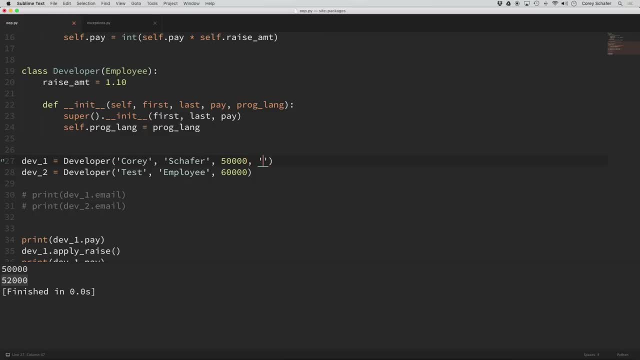 expecting a programming language to be passed in. So I'm just going to go ahead and pass in Python for our programming language. So I'm going to go ahead and pass in Python for our first developer and I'll pass in Java for our second developer. So now to make sure that this 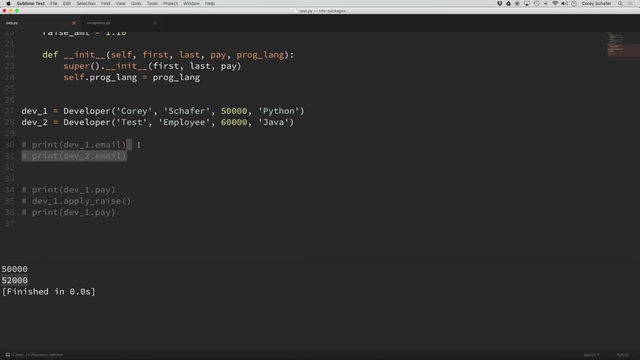 worked. I'm going to comment out those lines there and I'm going to print out the first developer's email and I'm also going to print out the first developer's programming language. Okay, so if I run that, then you can see that both of those were set correctly. So we got the 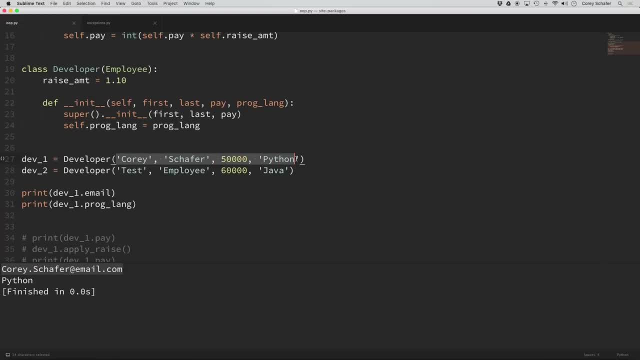 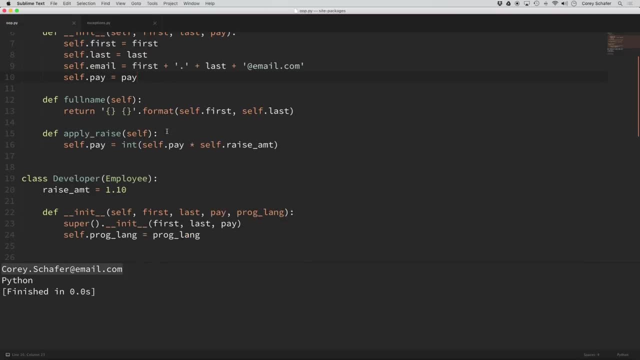 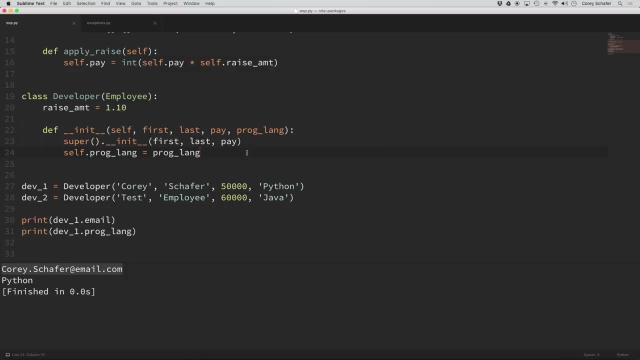 email set by it. When we passed in all of our arguments here, it came up here and it ran our employees init method and set all of those within there, And then it also set our programming language within our developers init method there. So you can see why this subclassing is useful. 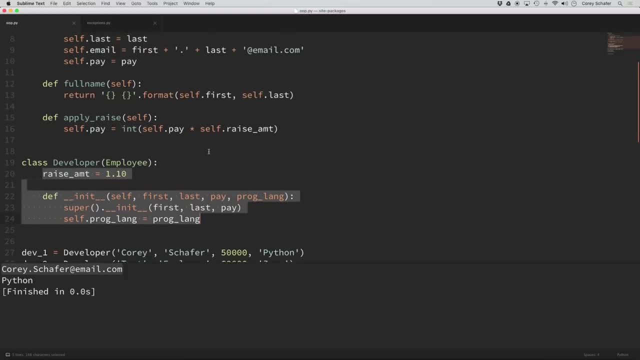 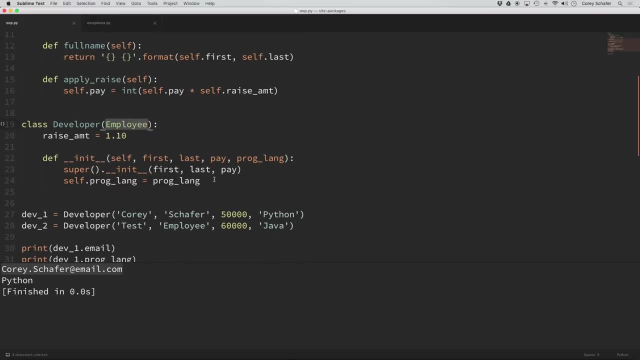 because we were able to customize just a little bit of code and we got all of this code from our employee class for free, just by adding in that one little line there. Okay, so, just so we can get a really good understanding of this, let's go through the process of creating another subclass called 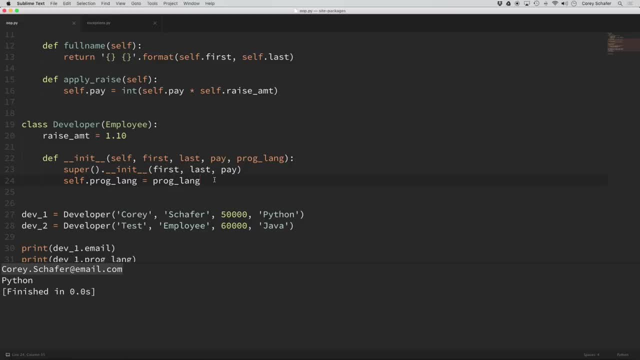 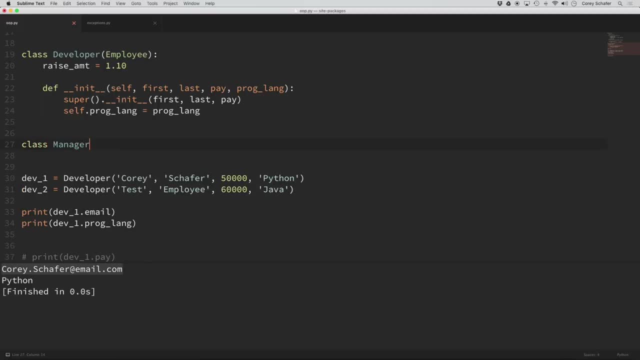 manager, And I'll go through all these steps again, but I'll go a little bit faster this time. Okay, so right here below our developer, I'm going to create another class and I'm going to call this class manager, And this is also going to inherit from employee. Now, when I create a new 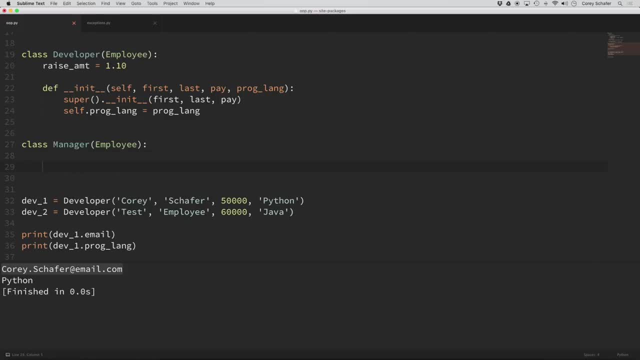 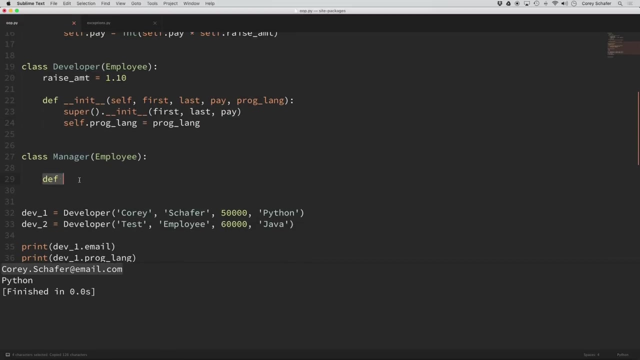 manager, I'm going to give the option of passing in a list of employees that this manager supervises. So we're going to need to add an init method for our manager And instead of typing all this in, I'm just going to grab this init method here from our developer and paste this in here. 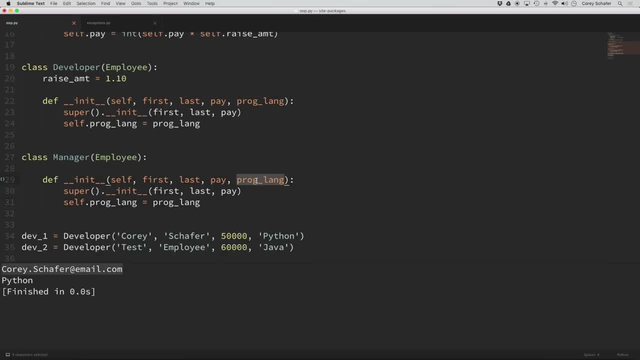 Okay, but this is going to be a little bit different. Instead of a programming language for our manager, I'm going to let them pass in a list of employees and I'm going to set the default to none. And then, instead of setting this programming language here, I'm going to say: 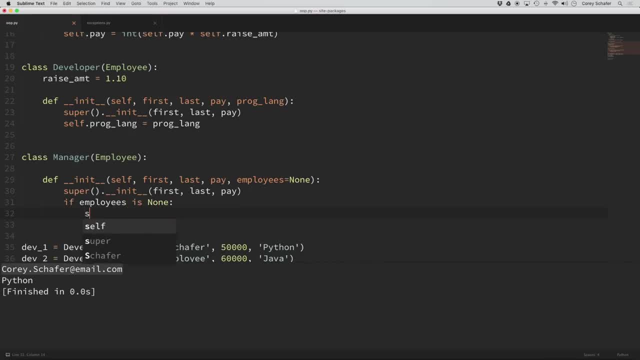 if employees is none, selfemployees is equal to an empty list, And then else selfemployees equals employees. Now you might be wondering why I didn't just pass in an empty list as default argument here instead of none. But you never want to pass mutable data. 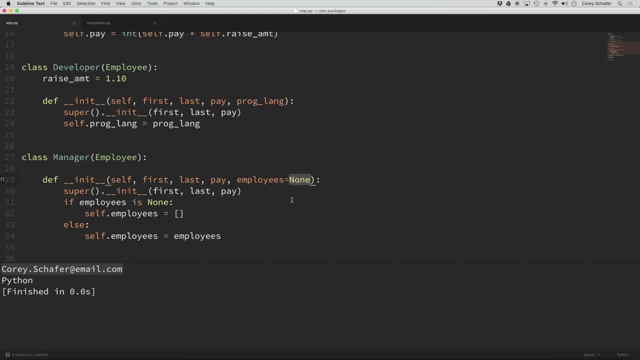 types like a list or a dictionary as default arguments, And that's a topic for another video And I plan on doing one on that soon. But for now, we'll just go ahead and set our employees to an empty list if the argument is not provided. And that's it for this video, If you have any. 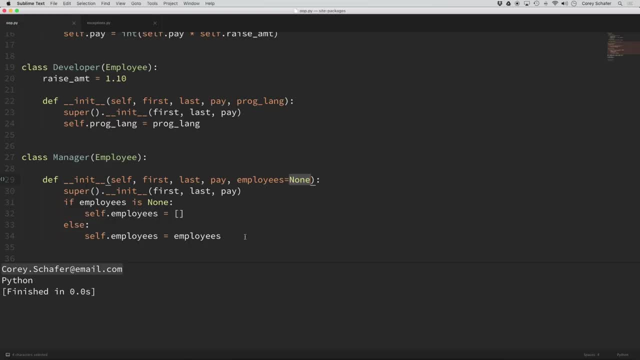 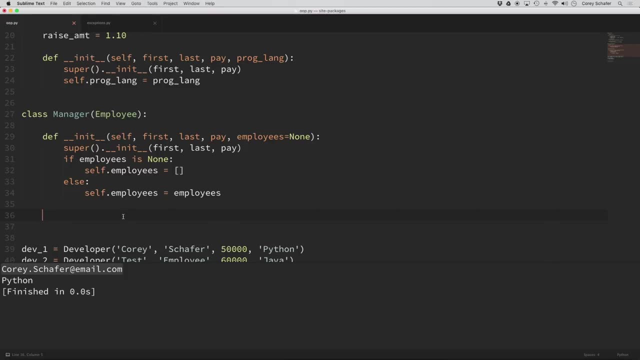 questions, feel free to leave them in the comments below And I'll see you in the next video. Okay, so now let's add in a few methods here. So I'm going to give the option to add and remove from our list of employees that our manager supervises, And to do this, I'll add in a method. 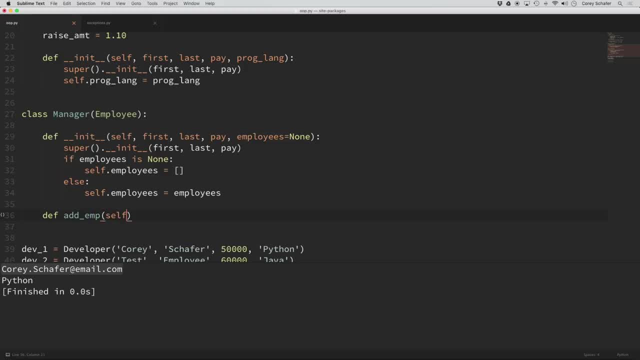 called addEmployee, And addEmployee will take self, just like all of our instance methods do, and employee, And then I'll just say: if the employee is none selfemployee, And then I'll just say: if the employee is none selfemployee, And then I'll just say: if the employee is none. 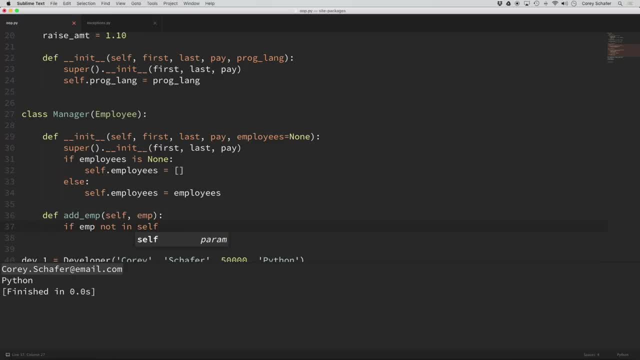 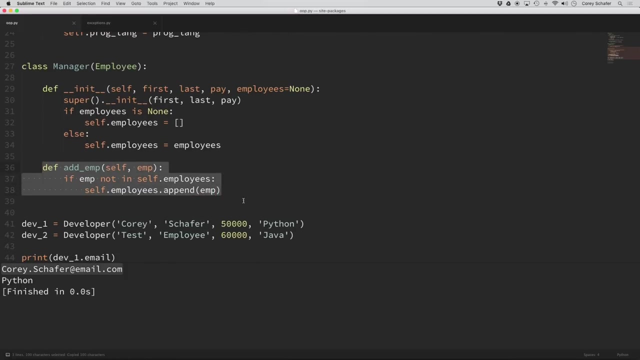 employee is not in selfemployees, then I will just append that employee to our list. So selfemployeesappend that employee. And now I'm also going to create another method here to remove employees from this list, And it's going to be similar, So I'm just going to go ahead and copy. 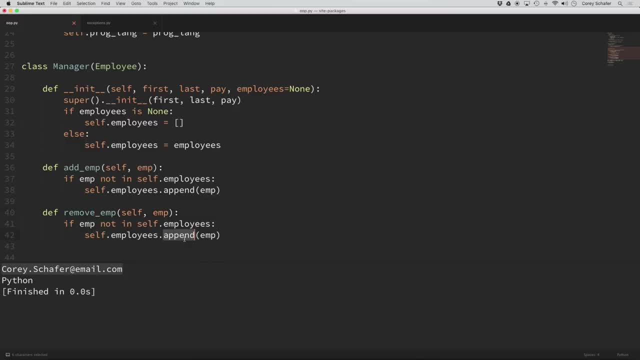 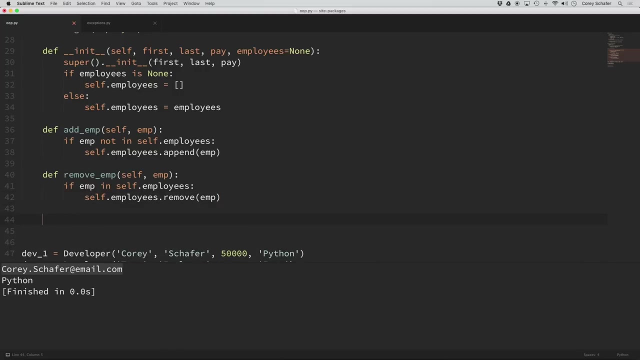 that, But this is going to be remove And we'll say: if the employee is in our list of employees, then remove that employee. Okay, and lastly, I'm going to add a method that will print out all of the employees that this manager supervises. So I'm going to call this method print employees. 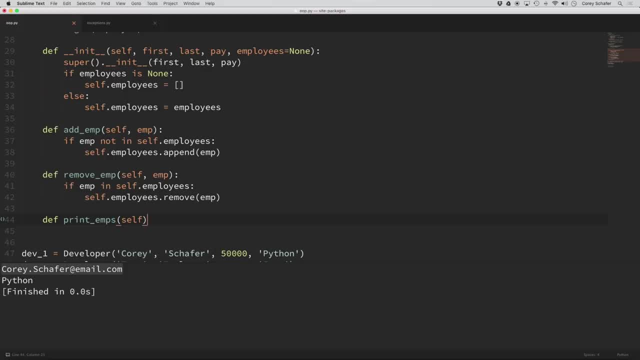 and this isn't going to take any more arguments than just self, and I'll say for employee in self, dot employees and then I will just print out that employee and before the employee I'll go ahead and put an arrow here, just so it sticks out a little bit further and instead of just printing the 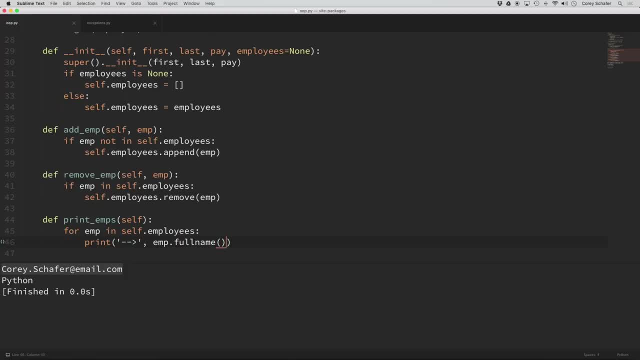 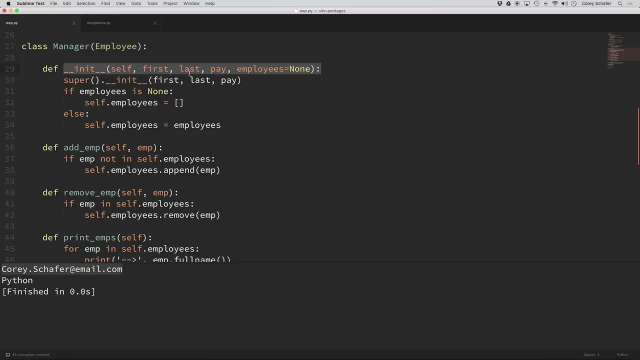 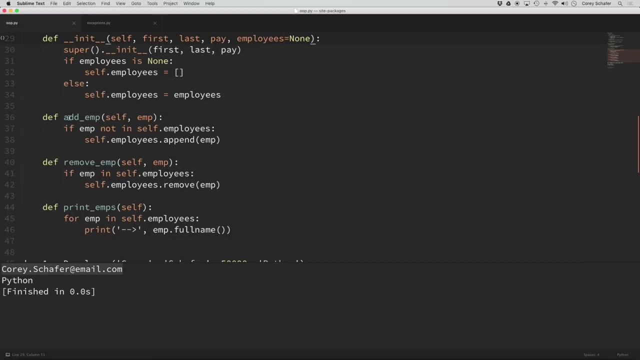 employee. I'll actually print out the employee full name. Okay, so I think that we are finished with our manager class. So we have our own init method here, which it'll accept: a first name, last name, pay and also a list of employees that this manager supervises, and then we 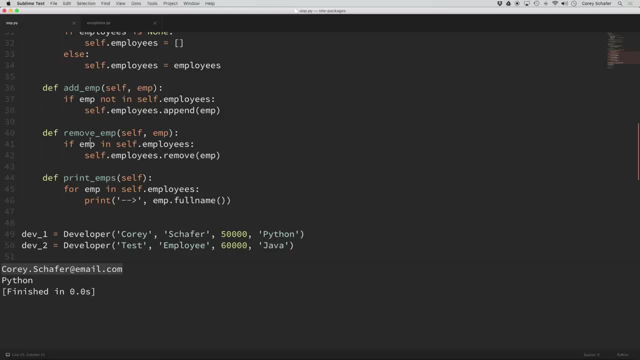 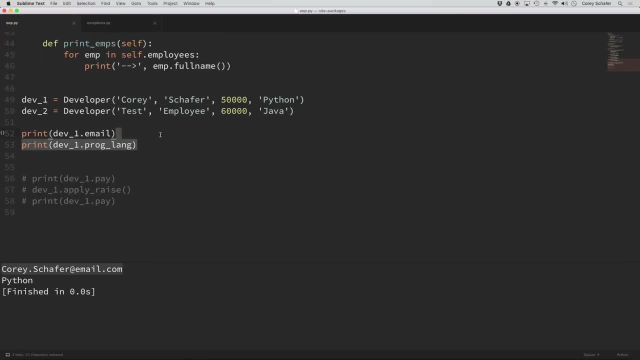 have a list of employees that this manager supervises and then we have a list of employees, the ability to add employees to that list, remove employees from that list and to print out all the employees from that list. So now let's see if this works. So I'm just going to comment out these: 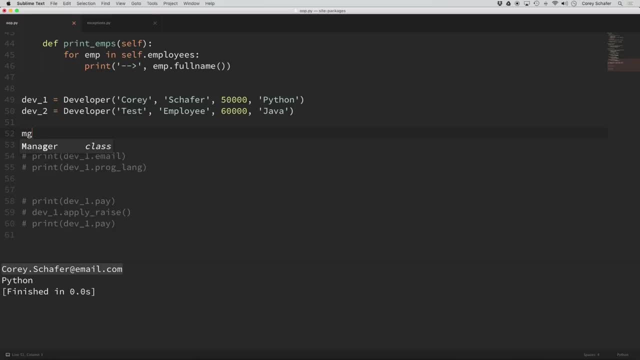 lines here and now I'm going to create a new manager and I'll call this manager one. So now I want this to be a manager, and for the first name, I'll do Sue, for the last name, I'll do Smith. We'll say that the pay is ninety thousand and let's say: 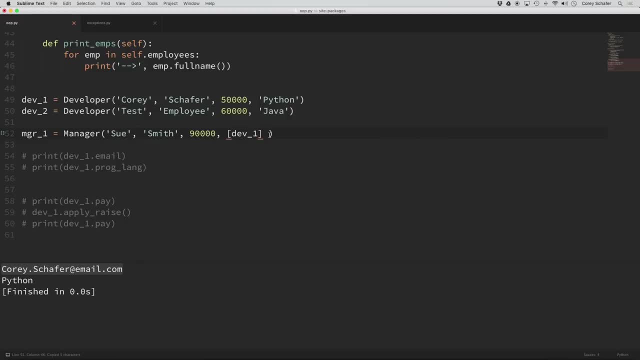 that she supervises this first developer here. So now let's make sure that this manager was successfully created and that we have all of the attributes and methods available that it would have inherited from that employee class. So let's go ahead and print out this: 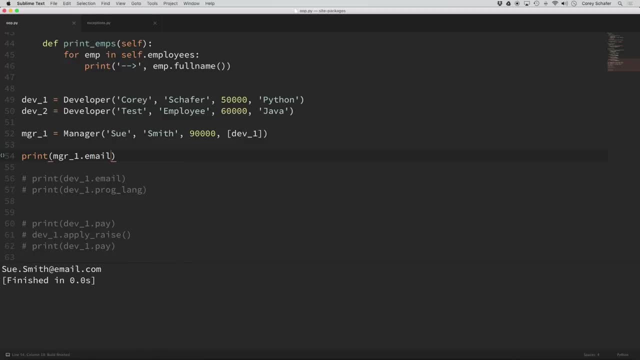 manager's email address. So now, if I go ahead and print this out, you can see that the email address was set correctly. But now we also added in all of this extra functionality. So let's see if we can print out all the employees that this manager supervises. So I'll do. 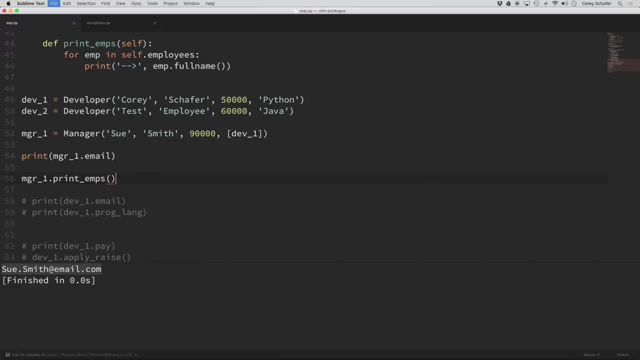 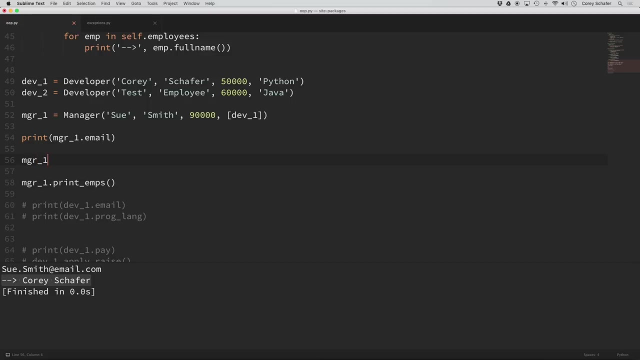 manager dot print employees and if I go ahead and run that, then you can see that it prints out the full name of the one employee that they currently supervise and I can add to that list of employees. So here I'll just say manager, one dot, add employee and I'll 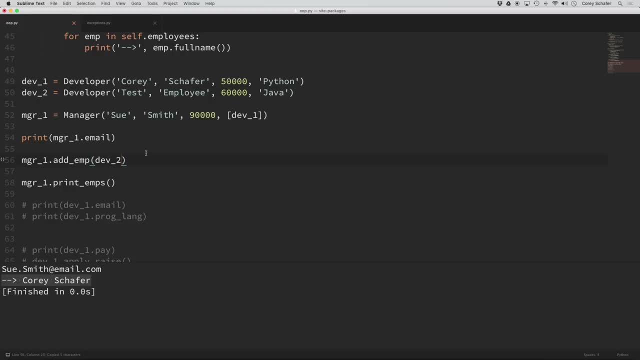 pass in this second developer Here before we print out that list of employees. Now, if I print that out, you can see that now they are supervising two employees and we also have the ability to remove employees. So I will remove our first employee here from their list of people who they supervise. So 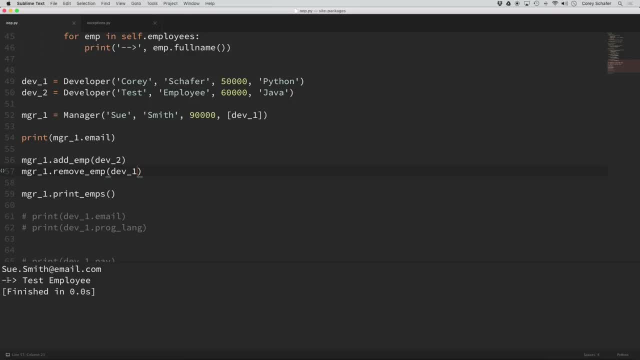 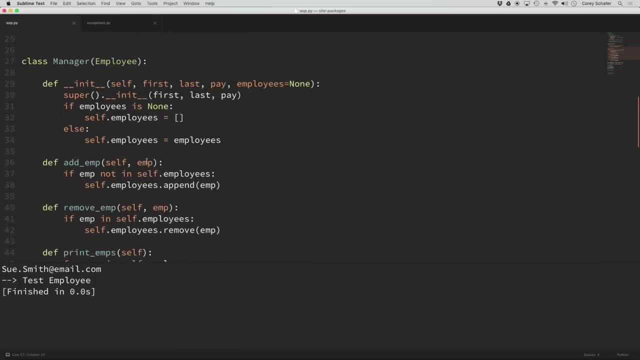 now, if I save that and run it, you can see that that first developer was removed from that list and they only have the second developer in that list. So, just like with our developer class, You can see how useful this actually is, because all of the code in here is specific to what. 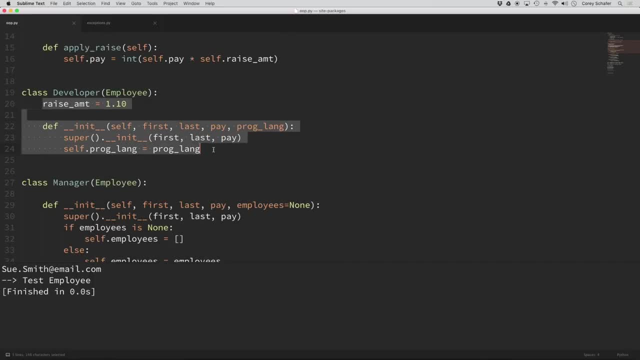 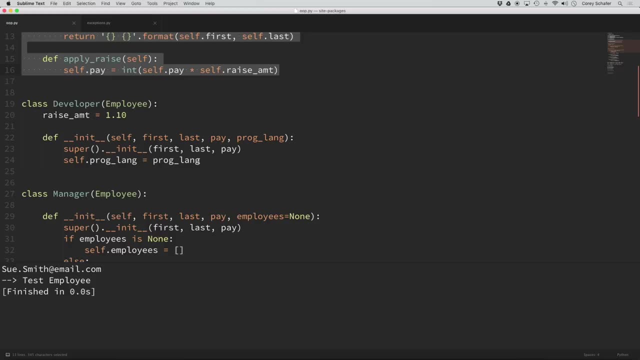 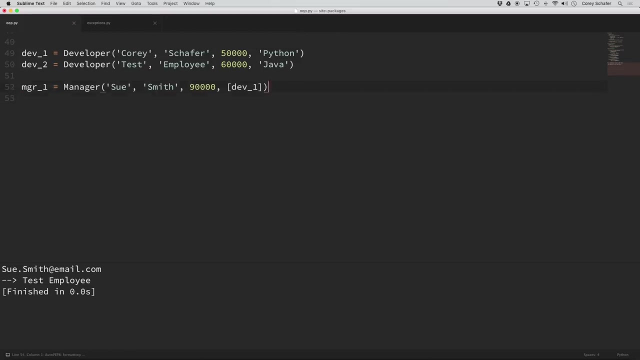 we want for a manager, and in our developer class it's specific to what we want for a developer, and we're inheriting all of this common code from employee, So we really get to reuse our code nicely here if we use subclassing correctly. Okay, so now I'm just going to go ahead and remove all of this code here. Now I know that. 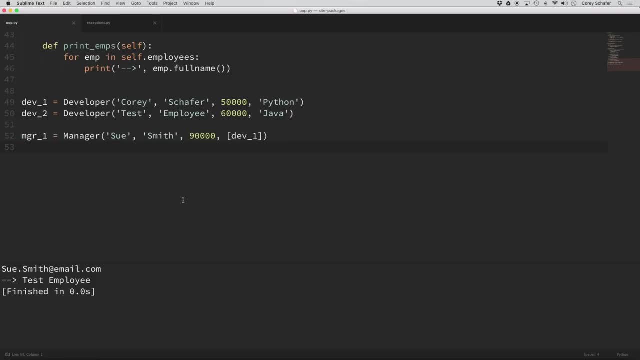 this video is getting a little long, but I want to show you a couple more quick things here. The first thing I want to show you is that the manager has these two built in functions called is instance and is subclass. So is instance will tell us if an object is an instance. 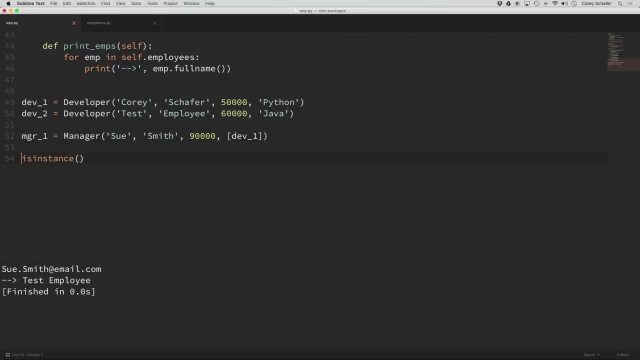 of a class. So, for example, if I need to print this out, I can print out whether manager one is an instance of manager, And if I print that out, you can see that it prints true. Now, if I was to check whether the manager is an instance of an employee, I'm going to 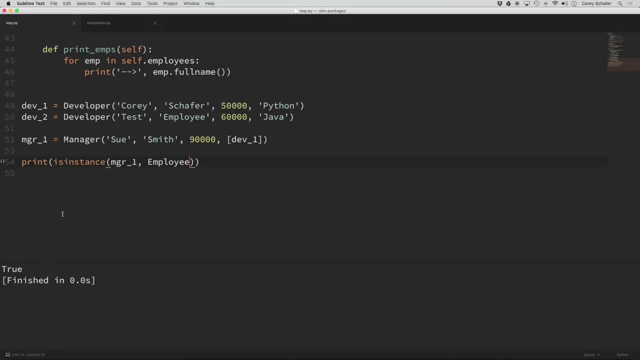 see that that is also true. But if I check, if manager one is an instance of a developer, then that returns false, because even though developer and manager both inherit from employee, they aren't part of each other's inheritance. So along those same lines we have. this is: 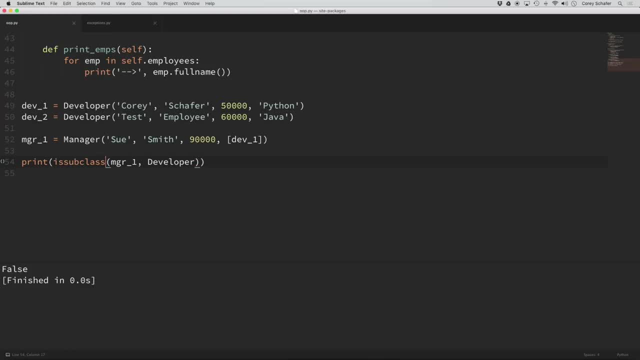 subclass function And is subclass will tell us if a class is a subclass of another. So, for example, I could do: Is a subclass of employee and if I run that, you can see that it returns true. and if I do, is manager a subclass of employee. if I run that, you can see that that. 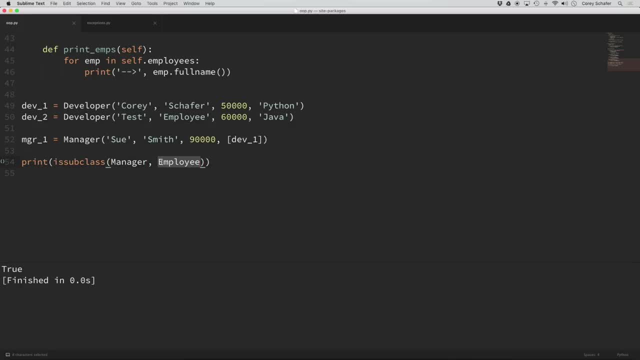 returns true also. but if I say, is manager a subclass of developer, then that will return false. so those built-in is instance and is subclass functions may come in use when you're experimenting with inheritance on your own, okay, so very last thing, I always like to show you all practical real. 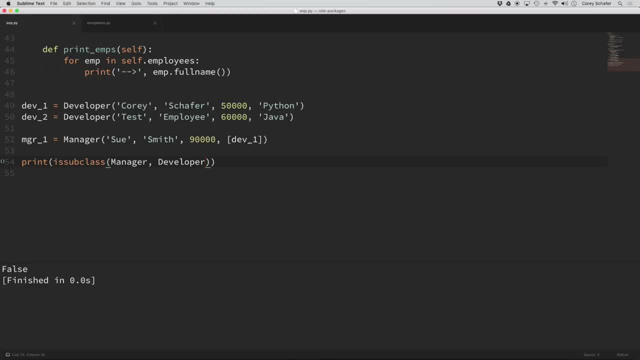 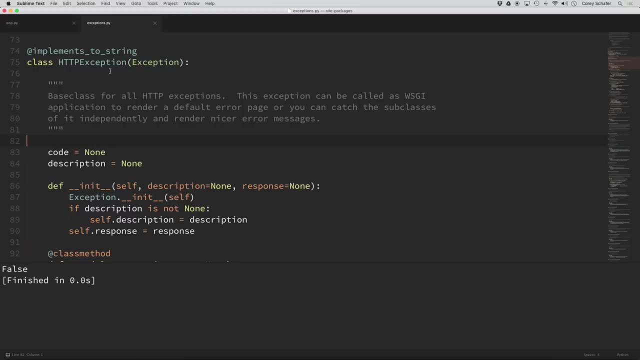 world examples of this stuff whenever I can, and one of the easier examples I found of subclassing was within the exceptions module of this Python whiskey library. so this is a really popular library and used in a lot of different projects. so if we look here, we can see that this HTTP exception class inherits. 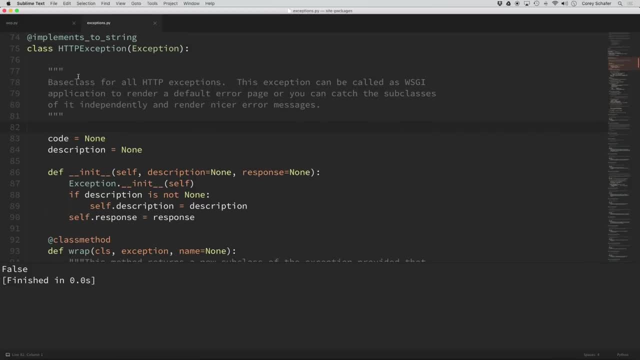 from this base exception and they say here that this HTTP HTTP exception exists in this base exception. and they say here that this HTTP HTTP exception exists in this base exception. and they say here that this HTTP HTTP exception exists in this base exception and they say here that this HTTP HTTP exception. 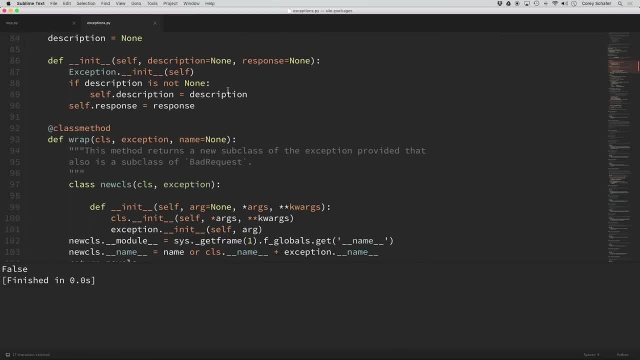 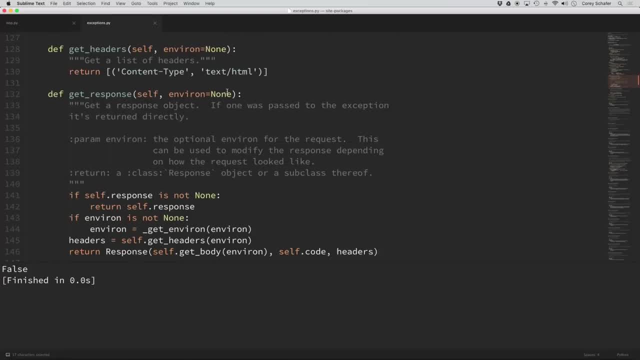 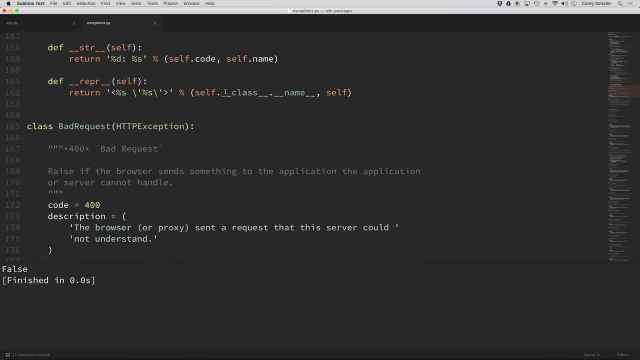